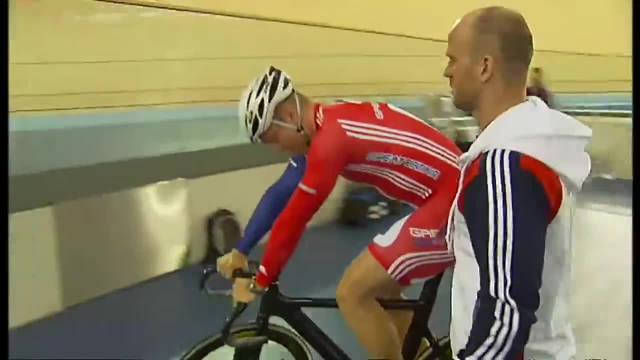 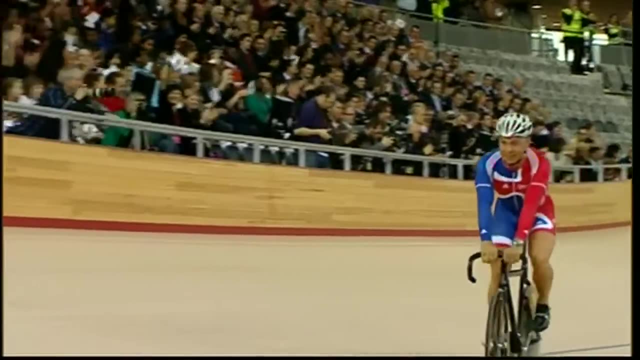 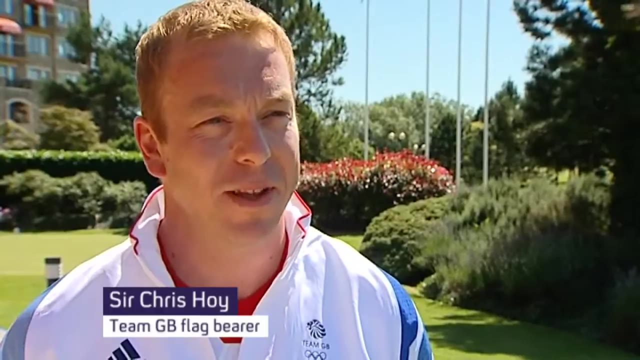 Sir Chris, who's won four Olympic gold medals in cycling, was given the honour after a poll of the British Olympic team And, despite his multiple medals and awards, he says this is his biggest accolade. I can't think of a bigger honour for an Olympian to be able to lead out the team into a home Olympics. 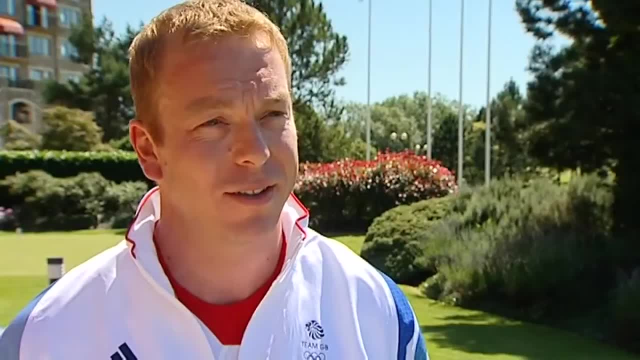 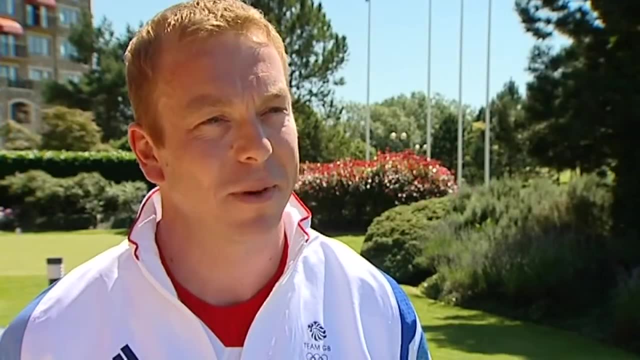 It really is something very special. You need a once in a lifetime opportunity. I was quite blown away when I heard the news yesterday to be voted by your fellow athletes. It means a great deal and I'm very much looking forward to the opening ceremony. 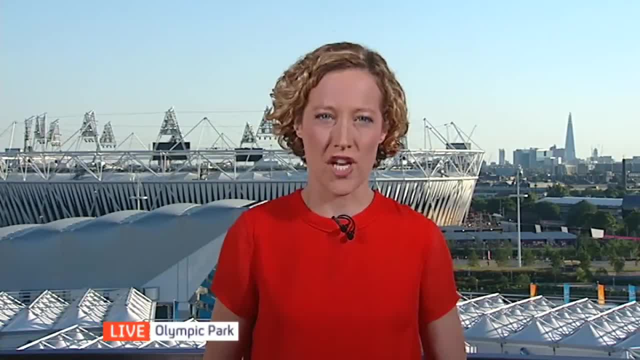 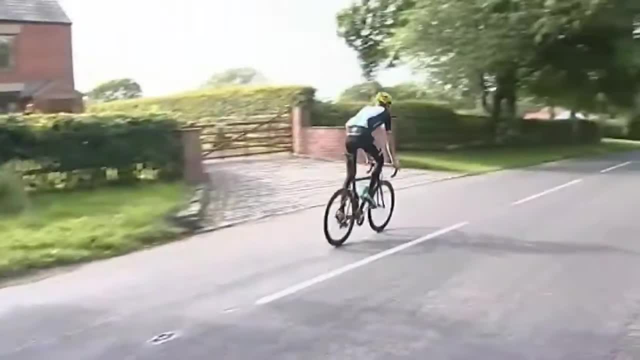 Well, Chris Hoy's team mate and Britain's first ever Tour de France champion, Bradley Wiggins, is back in the country to prepare for his Olympic challenge this weekend. Wiggins will spend a couple of days relaxing with his family before joining his cycling teammates on Wednesday. 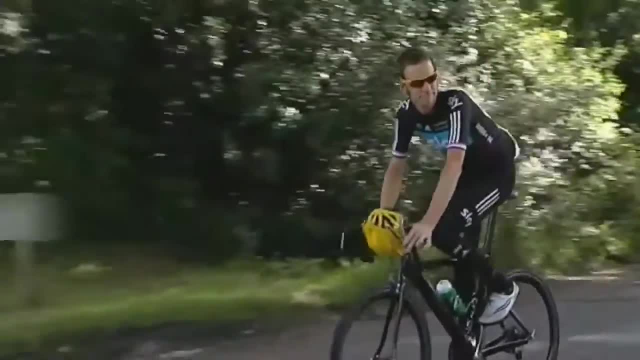 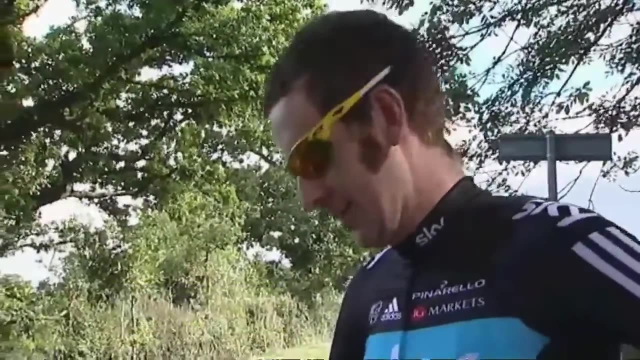 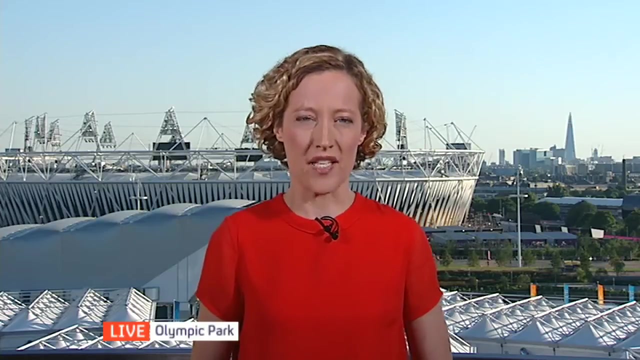 He says he's been simply overwhelmed by yesterday's victory. It's a little bit overwhelming. I didn't really expect all this And obviously I've seen a few of the papers today, So it's fantastic. It really is. So what happens if you turn up wearing a Pepsi T-shirt when one of the Olympics sponsors is Coca-Cola? 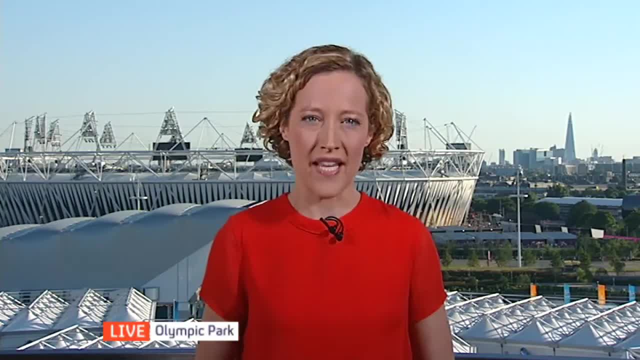 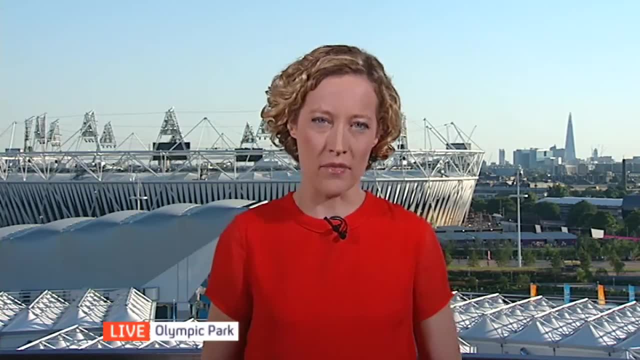 Well, the head of the International Olympic Committee says you will be allowed in, But there are incredibly strict rules in place to protect the companies who are paying £1.4 billion between them to sponsor the Games. So what exactly does all that money buy them? 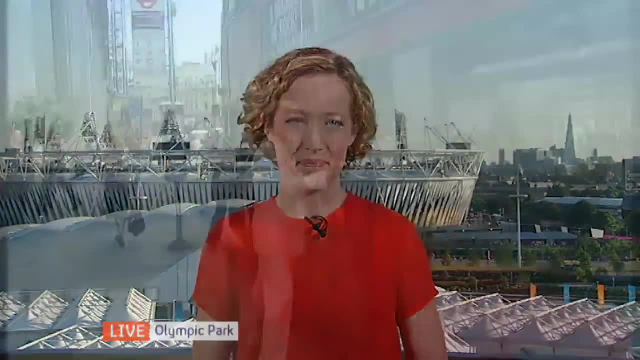 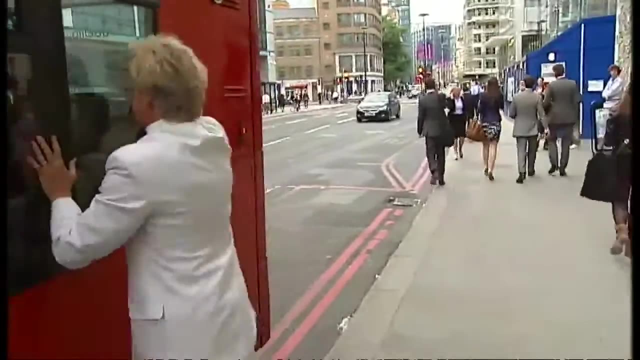 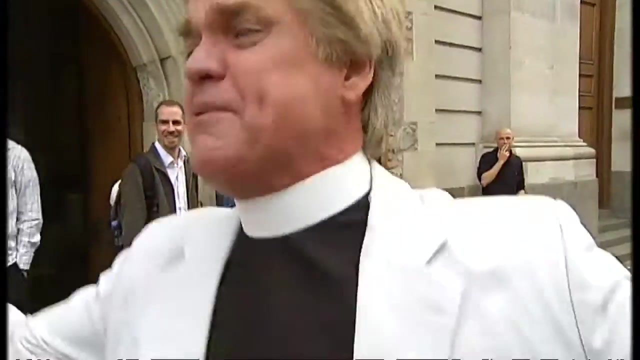 Our reporter, Porrick O'Brien, has been finding out. Get the corporations out of the Olympics, please. The Olympics are corrupt. Stop the sitting, Corporate sponsorship and the Olympics. It doesn't half get some people going. Reverend Billy Tallon is a comedian activist. 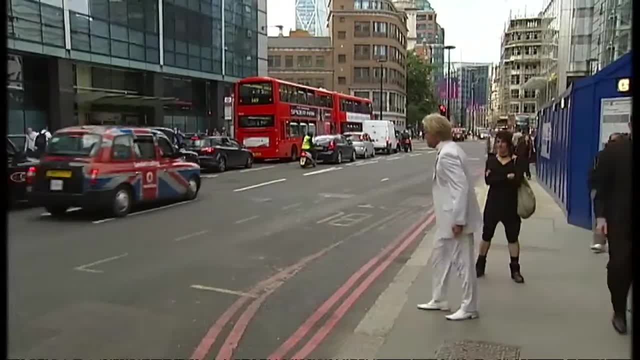 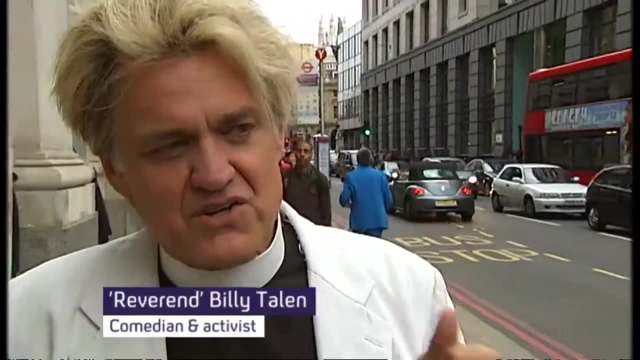 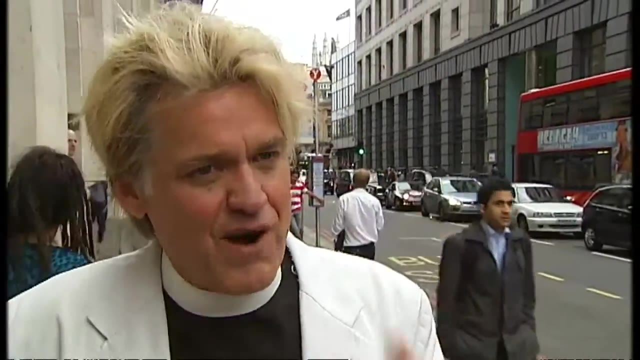 His character, an evangelical-style anti-consumerism preacher. This is the world coming together, So it has a very special, sacred human feeling And no, it should not be the grounds for corporations coming in. Amen, Praise be. 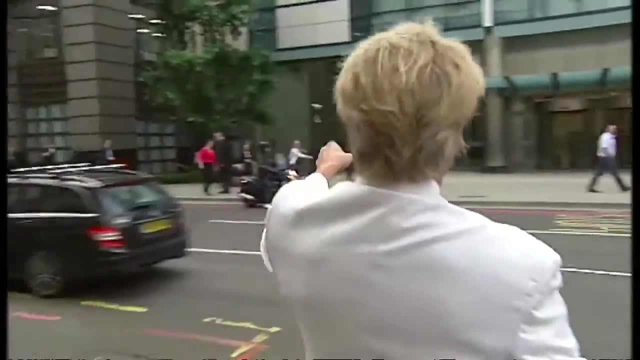 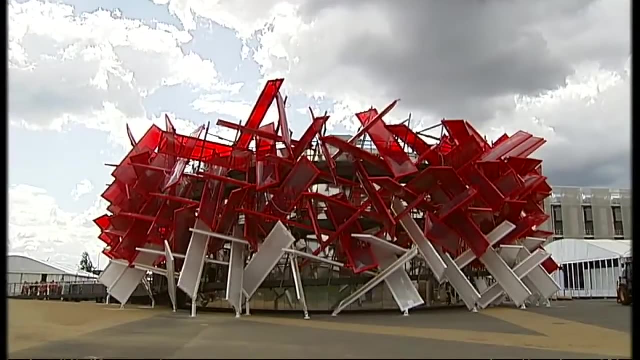 Do you work for a corporation? He was in London last week doing a gig At exactly the same time as this outburst. Coca-Cola's entertainment centre was being launched in the Olympic Village. Despite the hoo-ha, there's been over branding in the Olympics.